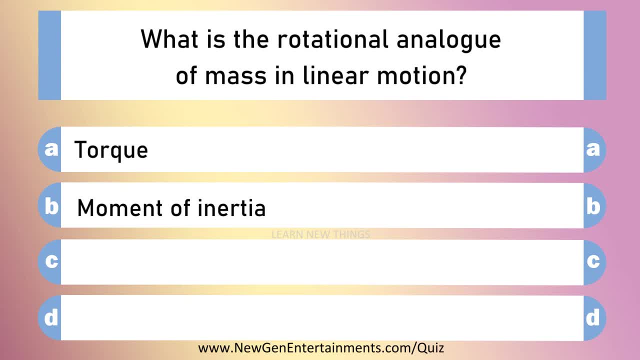 What is the rotational analog of mass in linear motion? Options are: A- Torque, B- Moment of Inertia, C- Angular Momentum, D- Weight. The correct answer is Option B- Moment of Inertia. What is the minimum escape velocity of a rocket to be launched from earth to space? 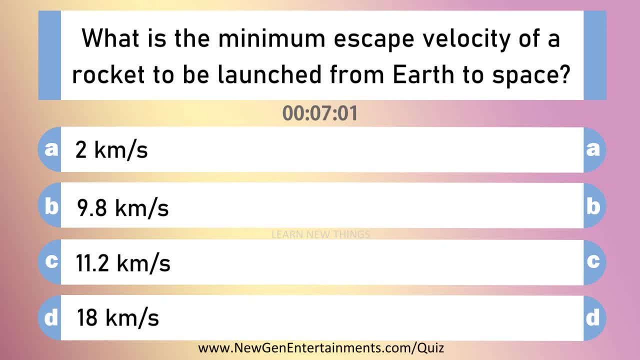 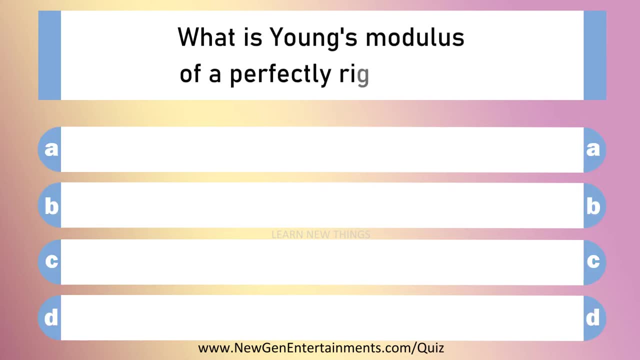 Options are: A- 2 km per second, B- 9.8 km per second. C- 11.2 km per second. D- 18 km per second. The correct answer is Option C: Moment of Inertia. What is Young's modulus of a perfectly rigid body? 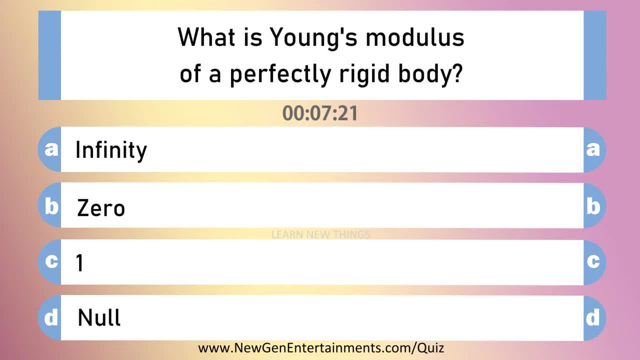 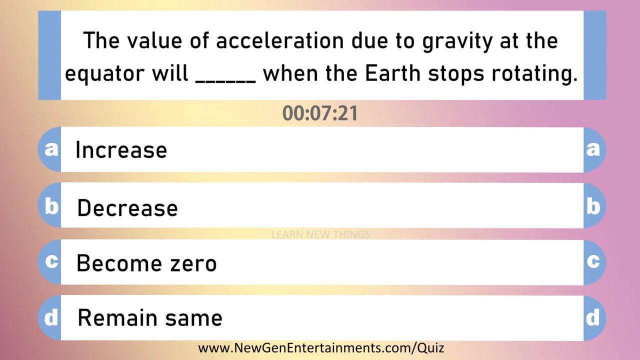 Options are: A- Infinity, B, 0, C, 1, D, Null. The correct answer is Option A, Infinity. The value of acceleration due to gravity at the equator will, When the air stops rotating? Options are: A- Increase, B- Decrease. 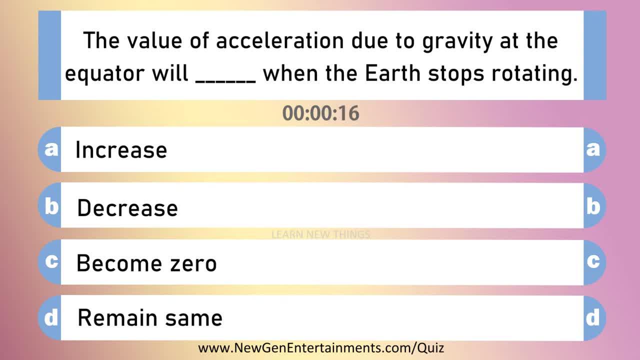 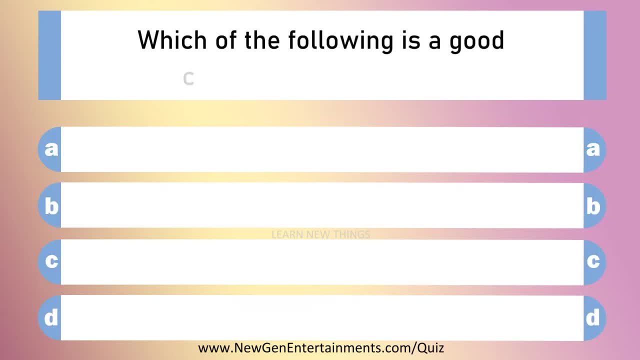 C- Become Zero and D- Remain Same. The correct answer is Option A- Increase. Which of the following is a good conductor of electricity? Options are A- Paper, B- Kerosene, C- Graphite and D- Dry Air. The correct answer is Option C- Graphite. 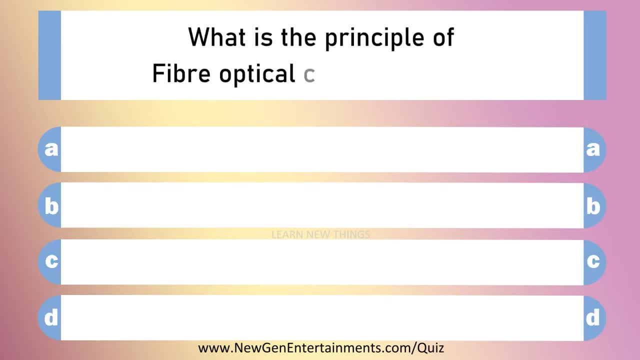 What is the principle of fiber-optical communication? Options are A- Interference, B- Scattering, C- Refraction and D- Total Internal Reflection. The correct answer is Option D- Total Internal Reflection. The correct answer is Option D- Total Internal Reflection. What is the frequency of direct current? 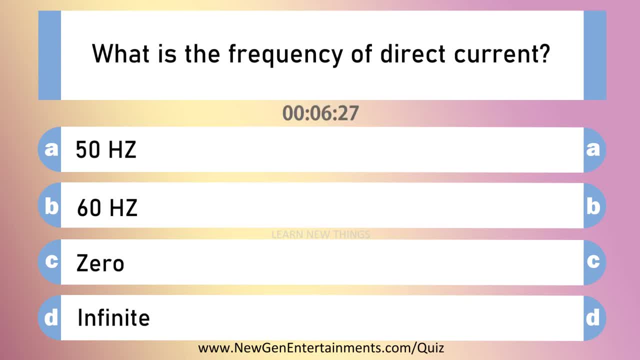 Options are: a- 50 Hz, b 60 Hz, c 0 and d- Infinite. The correct answer is option c 0.. Curie is a unit of Options: a- Temperature, b- Luminous intensity, c- Amount of substance and d- Radioactivity. 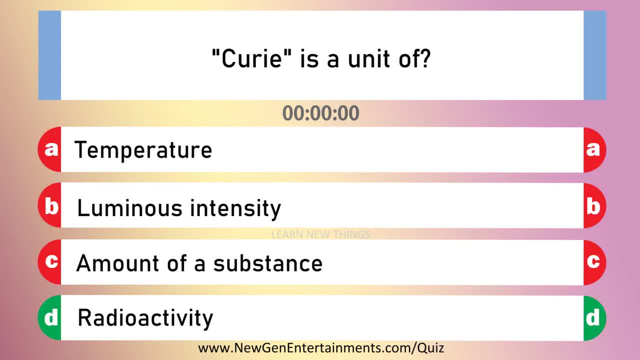 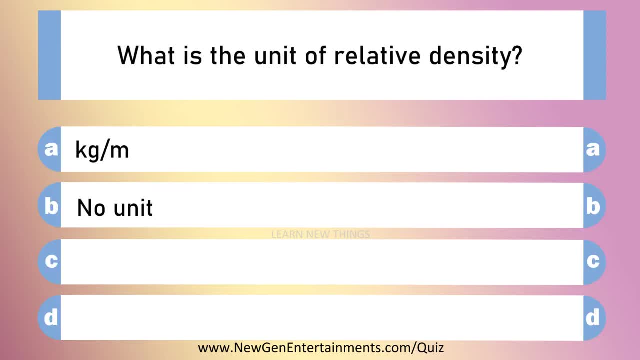 The correct answer is option d- Radioactivity. What is the unit of Relative density? Options are: a- Kilogram per meter. b- No unit. The correct answer is option c- Kilogram per meter square. d- Kilogram per meter cube. The correct answer is option b- No unit. 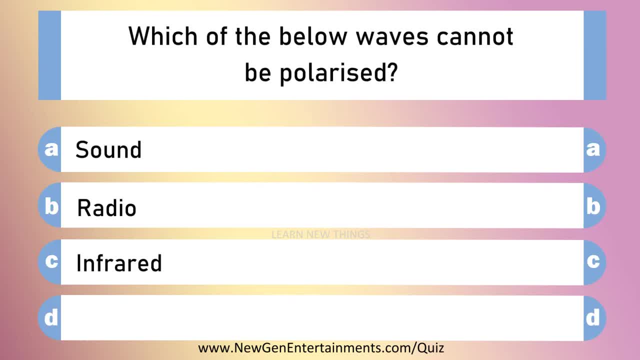 Which of the below waves cannot be polarized? Options are a- Sound, b- Radio, c- Infrared and d- Ultraviolet. The correct answer is option a- Sound. The correct answer is option d- Sound. What is the fourth state of matter? Options are a- Solid, b- Liquid, c- Plasma and d- Gas. 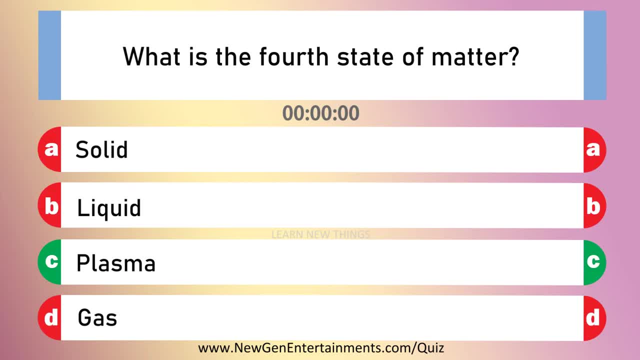 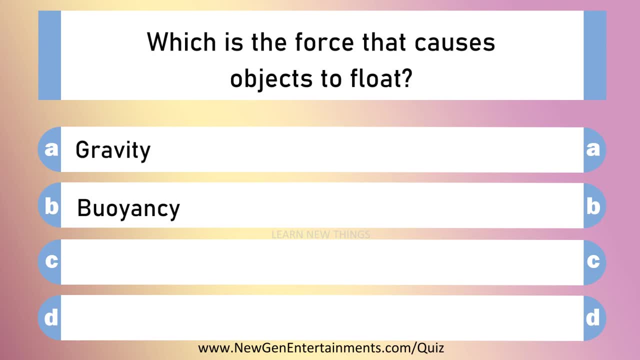 The correct answer is option c- Plasma, Which is the force that causes objects to float. Options are: a- Gravity, b- Buoyancy, c- Thrust and d- Friction. The correct answer is option b, Buoyancy. Which of the below is used to locate submerged objects? 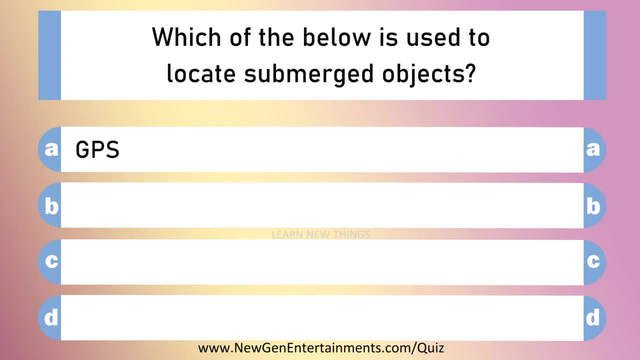 Options are: a- GPS, b- Anemometer, c- Sonar and d- radar. The correct answer is option c, Radioactivity. The correct answer is option d, Frequency. The correct answer is option c- Thermometer, d- Radar. The correct answer is option g, Arrival. 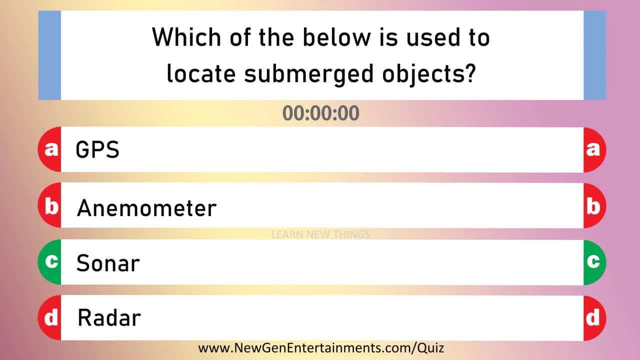 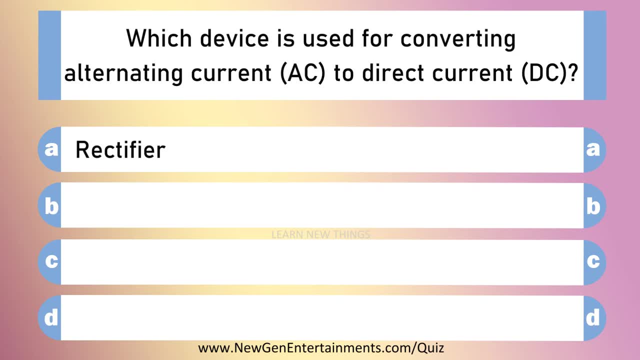 The correct answer is Option C- Sonar. Which device is used for converting alternating current to direct current? Options are A- Rectifier, B- Transformer, C- Dynamo and D- Induction Coil. The correct answer is Option A- Rectifier. 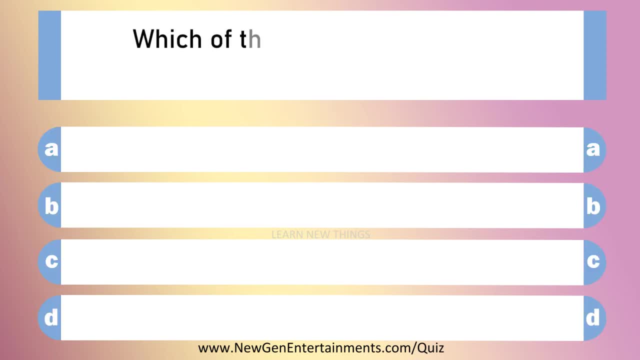 Which of the below is a measure of sound level? Options are A Celsius, B Becquerel, C Coulomb and D Decibel. The correct answer is Option D Decibel Acceleration is inversely proportional to. Options are A Force. 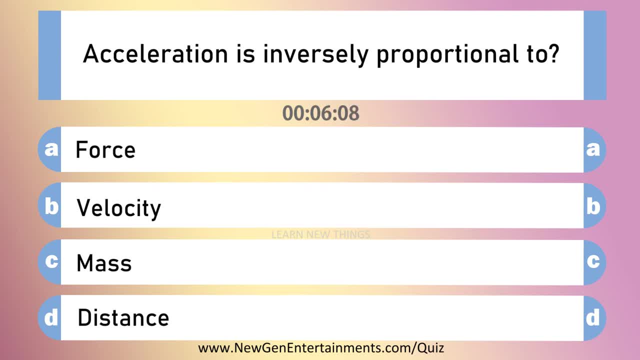 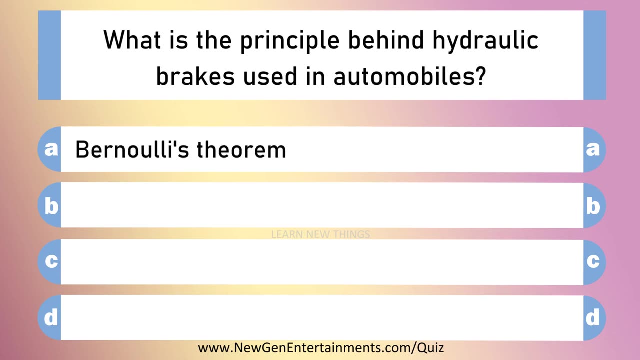 B- Velocity, C- Mass and D- Distance. The correct answer is Option C- Mass. What is the principle behind hydraulic brakes used in automobiles? Options are A Bernoulli's Theorem, B Pascal's Law, C Newton's Law and D Archimedes' Principle. 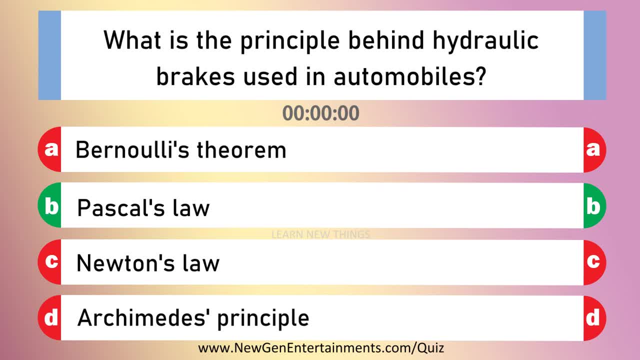 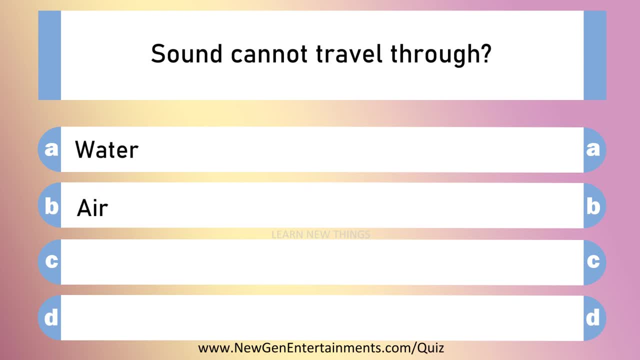 And the correct answer is Option B- Velocity. And the correct answer is Option B. Pascal's Law: Sound cannot travel through Options A- Water B, Air C, Vacuum, D- Metal. Conclusion: The correct answer is Option C- Vacuum. Changes in theArthur type of options. 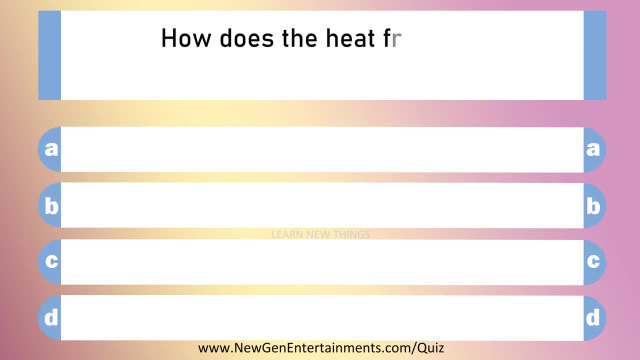 Appearance 3X M Earth. Options are A- Radiation, B Conduction, C Convection and D- Induction. The correct answer is Option A, Radiation. What is it called when the Sun is exactly over the Earth's? 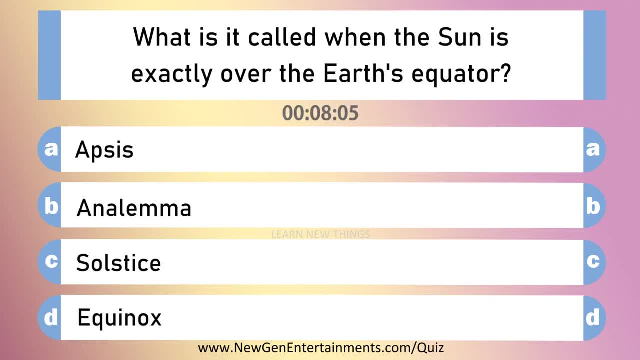 equator. Options are A- Apsis, B Analemma, C- Solstice and D- Equinox. The correct answer is Option D, Equinox. The surface tension of a liquid decreases when its temperature is. Options are A- Increased, B Decreased, C Unaltered and D- Zero. 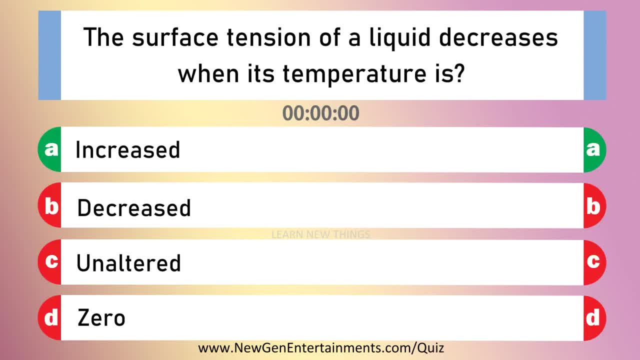 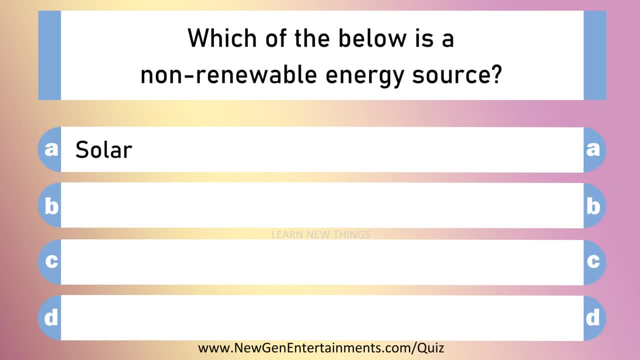 The correct answer is Option A- Increased. Which of the below is a non-renewable energy source? Options are A- Solar, B- Wind, C- Fossil Fuels and D- Tidal. The correct answer is Option C- Fossil Fuels. 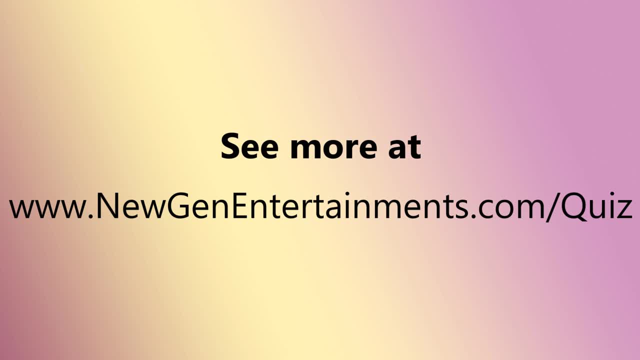 The correct answer is Option A- Solar, B- Wind, C- Fossil Fuels and D- Tidal.